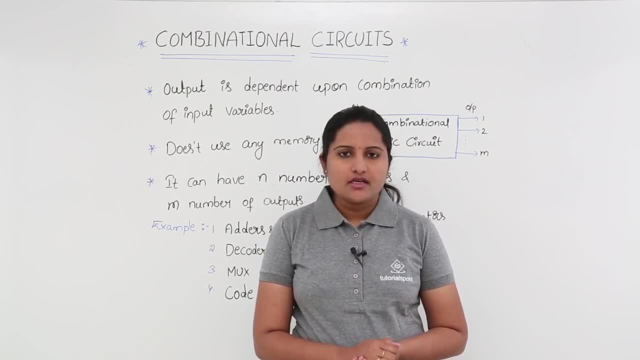 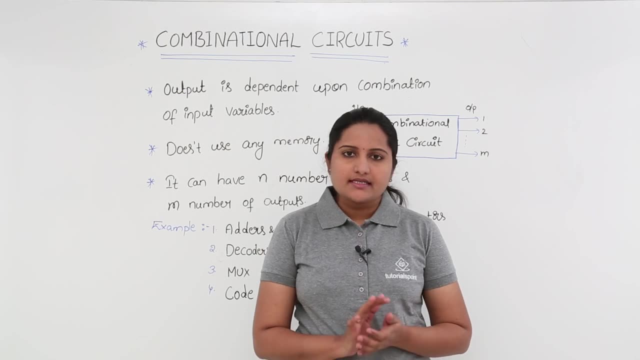 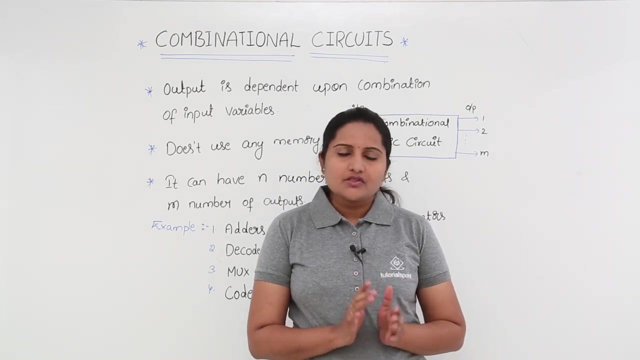 In this class we are going to discuss about combinational circuits. So generally, combinational circuit is a circuit whose output will depends upon the input variables. As the name indicates, the output of a combinational circuit will depends upon the combination of input variables given. So generally, this is a logic circuit which is having different logic. 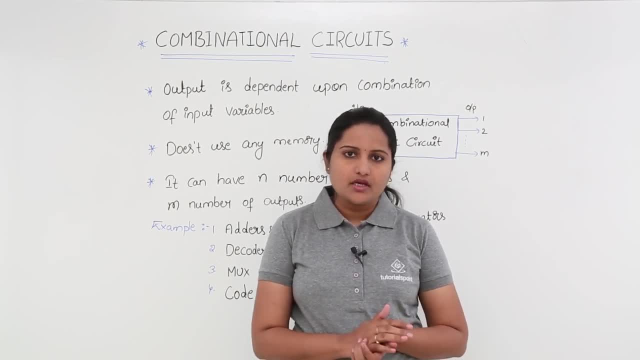 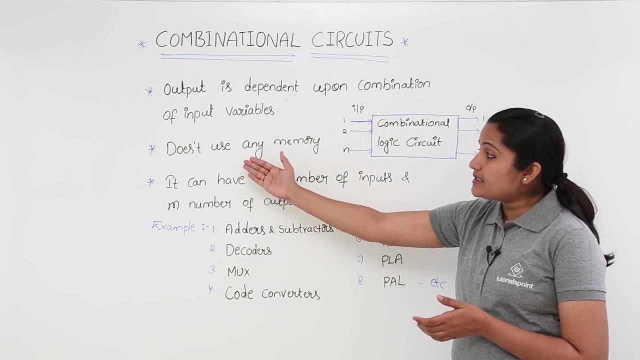 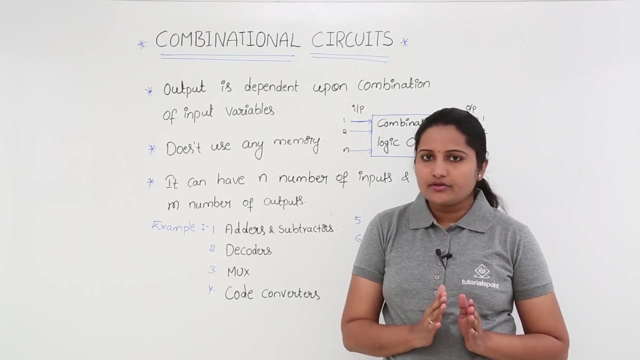 gates inbuilt in, integrated in a circuit. So see here, the output is dependent upon combination of input variables and it does not use any memory, as this is only dependent upon input combination and it is not going to depend upon any previous state inputs or any other. 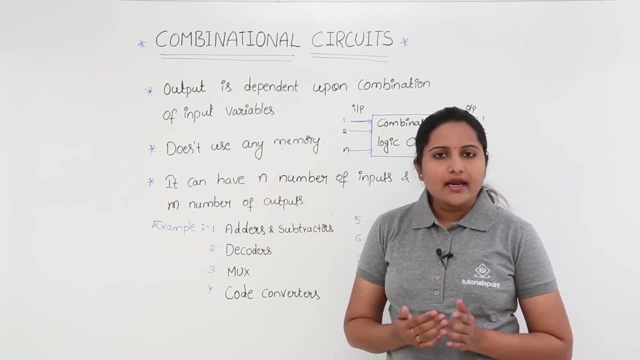 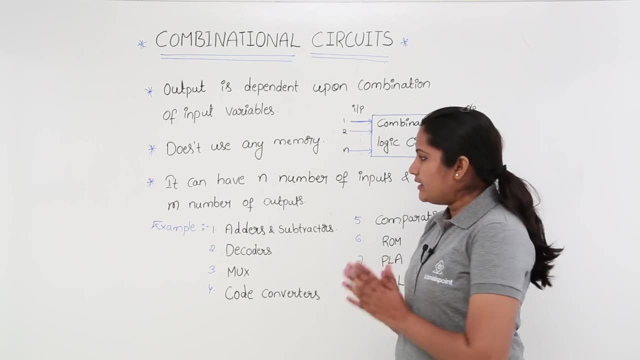 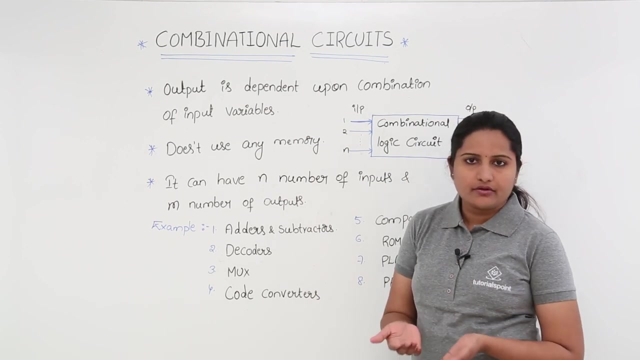 Here. it does not require any memory and previous state inputs would not have any effect on the output of this combinational circuit, and it can have n number of inputs and m number of outputs. That means you can have n number of inputs for your combinational circuit and you may have m number of outputs. 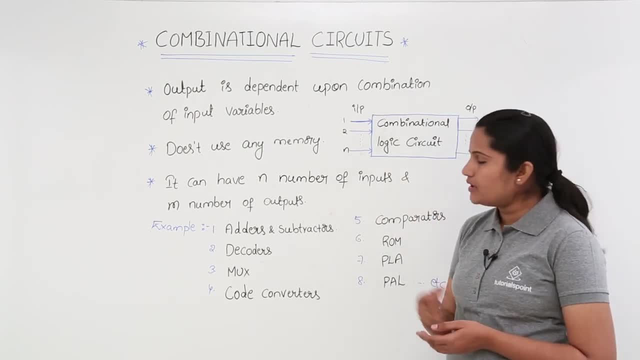 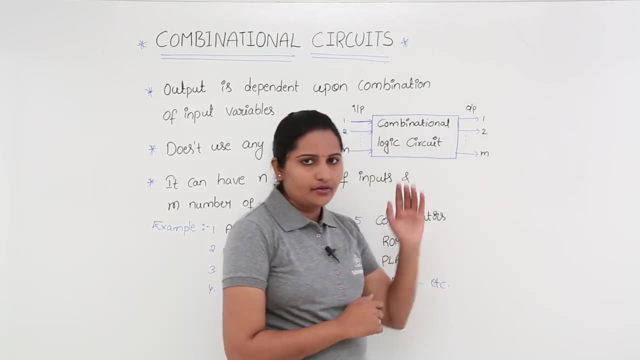 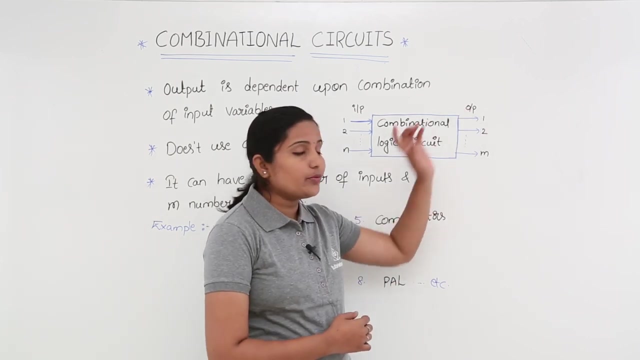 So this is the basic black diagram of a combinational circuit. Here you are watching n number of inputs and m number of outputs for this combinational circuit. Here the inputs are always called as excitations for combinational circuits and output is called as response of. 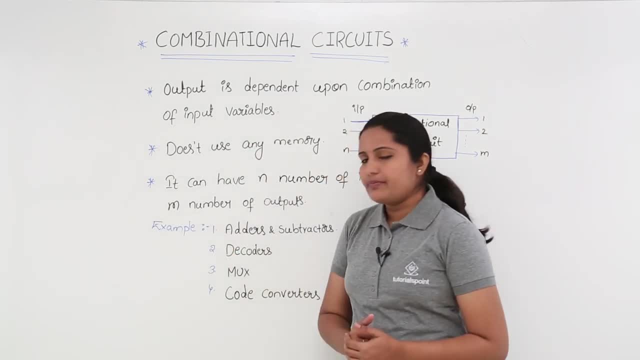 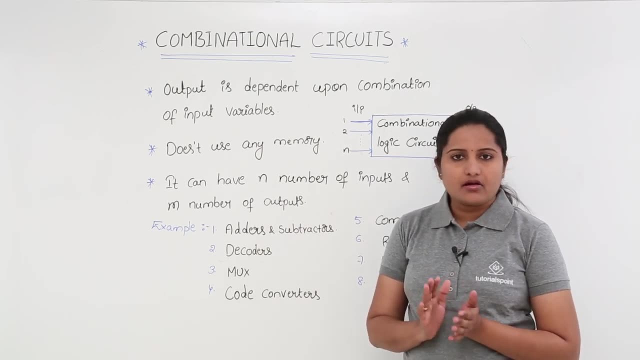 circuit. So here these are the best examples for combinational circuit. those are adders and subtractors, So these adders and subtractors, or binary adders and subtractors, and decoders, So which decodes input into output. So here multiplexes are there and code converters, which 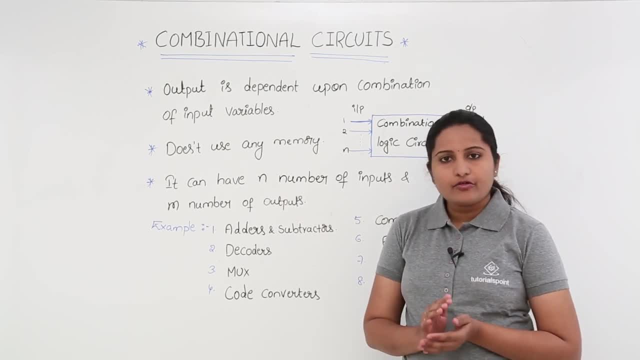 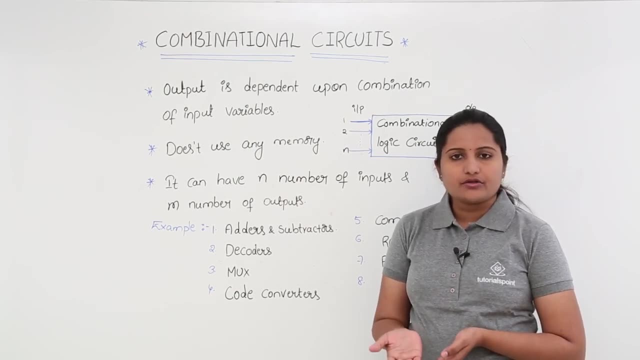 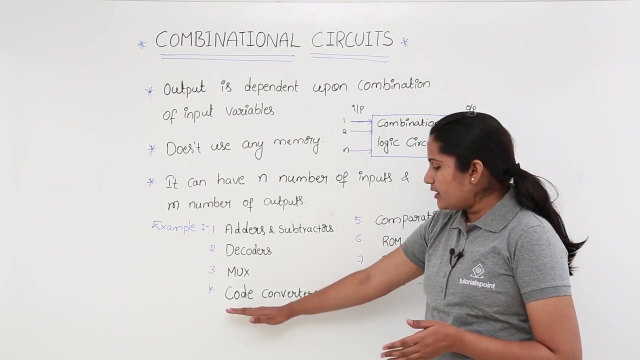 converts one code to another code, like, for example, if you want to convert BCD to binary, binary to BCD, BCD to gray code, if you want to design gray to binary. like that, If you want to convert one code to another code, you need code converters. These code converters are also an example of